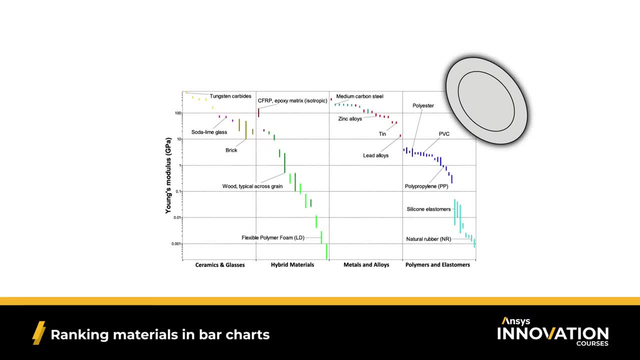 application like a dinner plate. I know I don't want a floppy dinner plate. Therefore, we want a material with a high Young's modulus, or to maximize Young's modulus. So we focus on the upper portion of our chart. But what if I'm instead designing a material for the 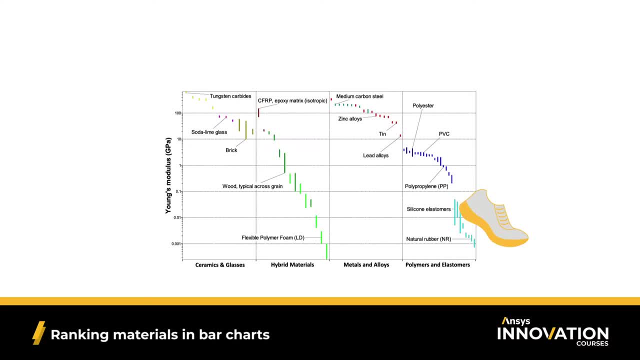 bottom of a running shoe. I want some amount of stiffness, but in order to protect my joints, I need something with a lower stiffness than my dinner plate. Therefore, I'm going to shift my focus lower on this bar chart And look to optimize my property in this region, Once again using a logarithmic scale here. 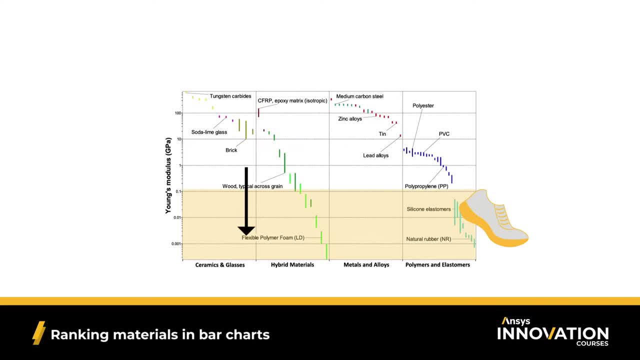 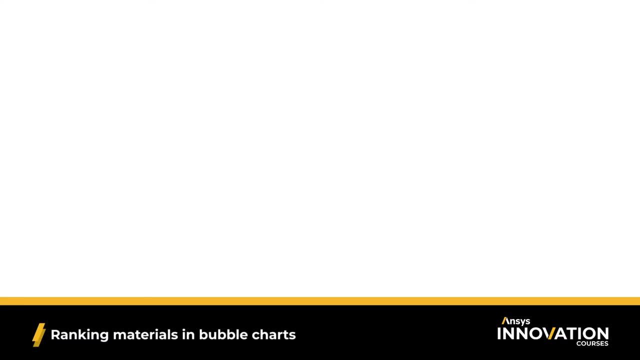 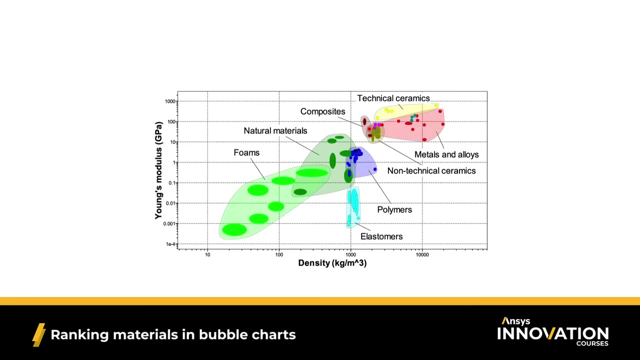 instead of linear is very useful to help make the ranking process easier to visualize. Well, comparing one property is just fine, but design usually requires considering more than one property. We can use our bubble charts to compare two material properties against one another. Here things are a little more complex than with our bar charts. 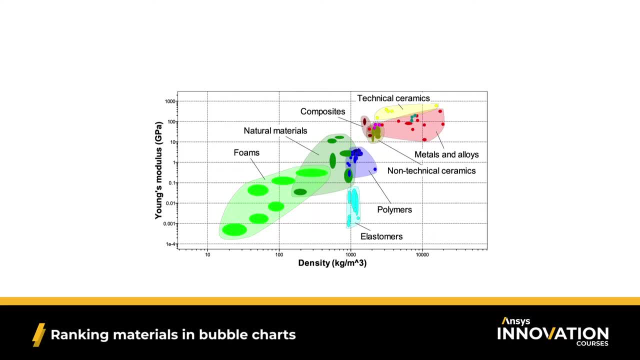 Our example here is a Young's modulus versus density bubble chart. Remember, the small ovals and circles represent individual materials, while the larger envelopes show material families. We can think about this chart in four quadrants. So if we start in the lower left corner, we 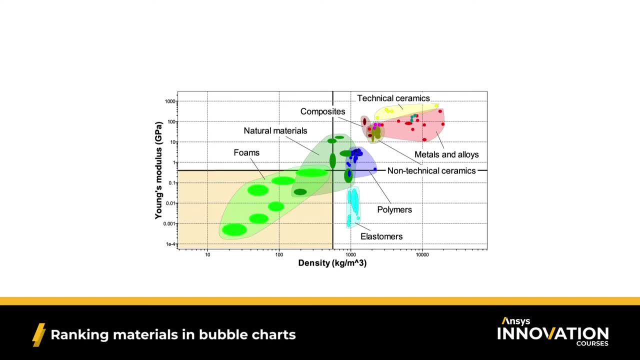 can see materials that have low stiffness and low density Makes sense. we're seeing our foams, particularly polymeric foams, in this corner. Again, depending on our design criteria, we either want to focus on this quadrant or avoid it. 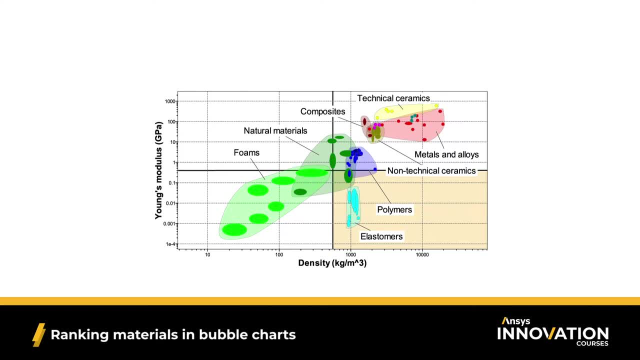 Next we have the lower right corner, where we have low stiffness but high density. Notice how there aren't a lot of materials in this quadrant. We have some elastomers and that's mostly it. This is okay, as generally a structural design doesn't need a heavy yet not very. 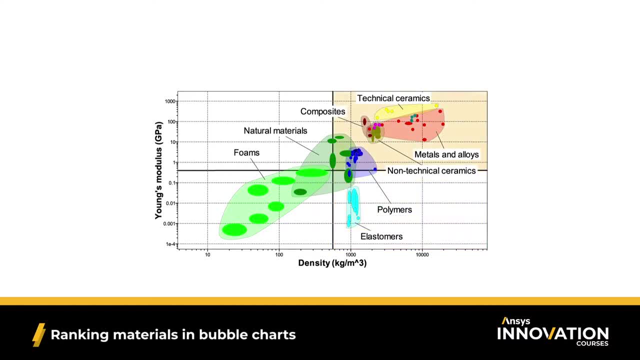 stiff material. Next we move to our upper right hand corner, where we have high density and high stiffness materials. Our technical ceramics and metals can be found here, with composites sitting right at the edge. Finally, we have the upper left hand corner. Once again, it's mostly empty, apart from 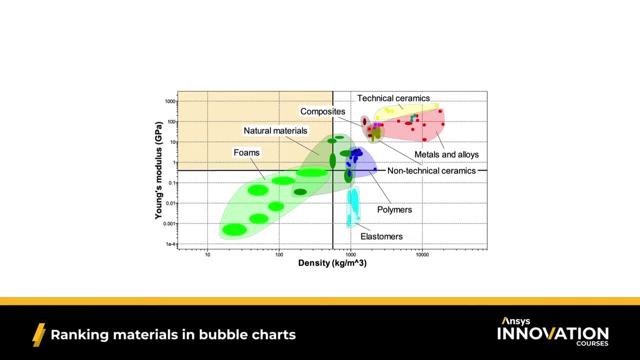 our composites. Many engineers and designers consider this quadrant filled with the ideal materials: High stiffness but low density, Perfect for aerospace and automotive applications. While no materials really exist up here, especially in the middle, Our property charts can help us pick materials close to this ideal as possible. It also allows 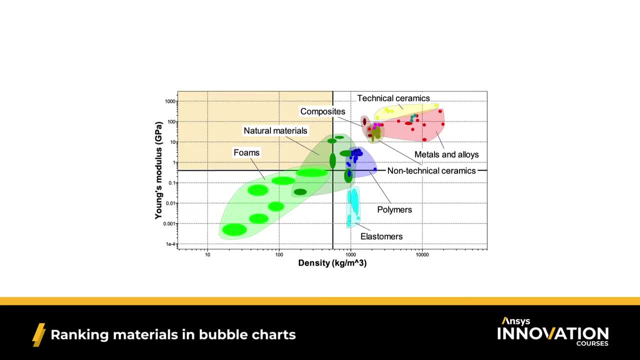 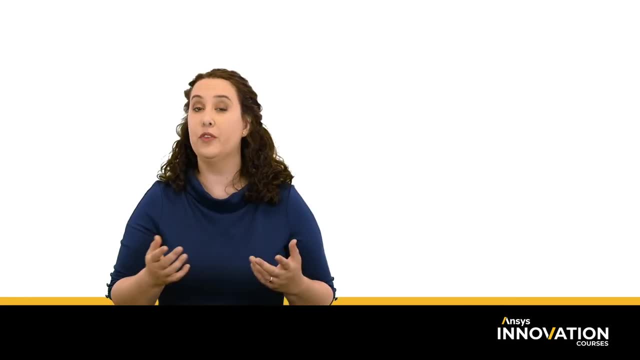 material scientists and designers to see how brand new materials can fit within the landscape of existing engineering materials. So we've now seen how we can use our property charts to help us rank our materials based on our design criteria. But the charts I showed you only have about a hundred engineering 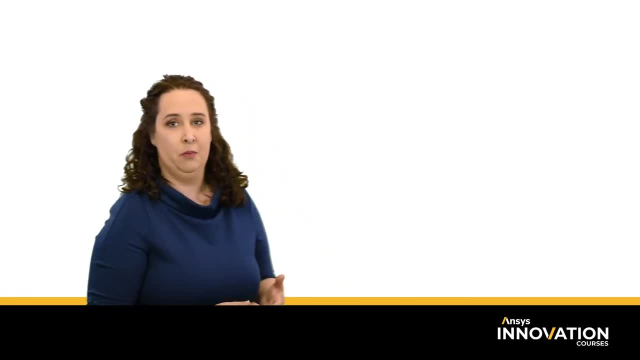 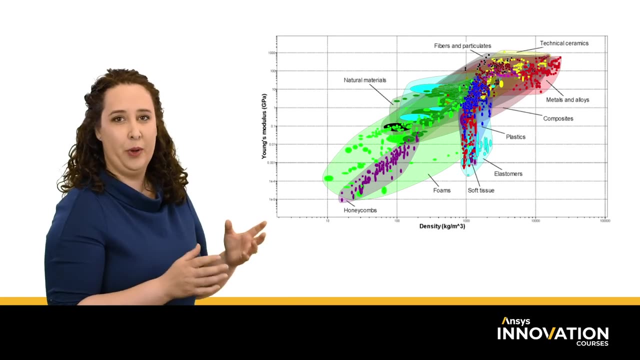 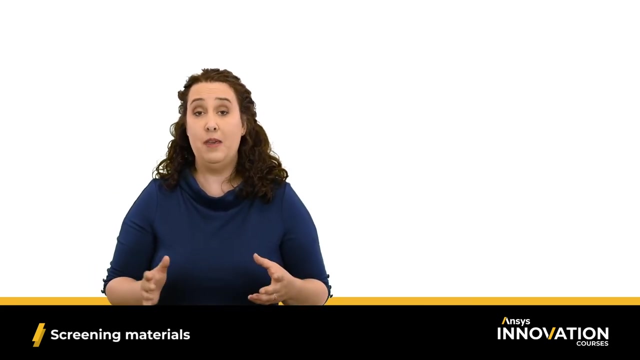 materials. In reality, we have thousands of engineering materials, So our chart should really look something like this: This is so much more information to sort through. Is there some way that we could simplify this? Well, we can go back to our design criteria. Maybe there are some material families that. 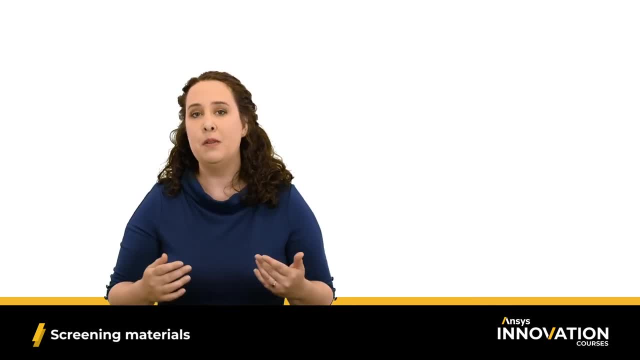 I just don't need to consider, Or maybe I have a minimum acceptable value for a specific material property, so I can simply toss out the materials that don't meet that minimum. This process is called screening. It actually occurs before ranking. Screening means I'm tossing out unsuitable materials and then I rank the materials. 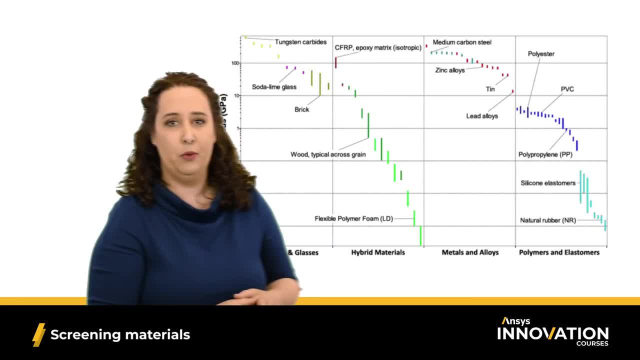 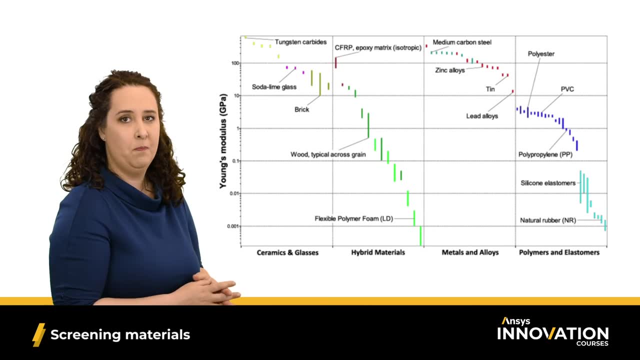 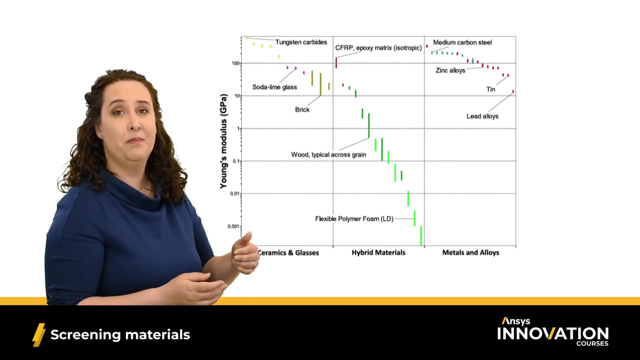 that are left over. So we can see this example in a bar chart. Here I have a bar chart of yield strength on my y and I've split the x-axis based on material family, Based on my design criteria. I know that I don't need to consider polymers and elastomers, so I can just get rid of them. 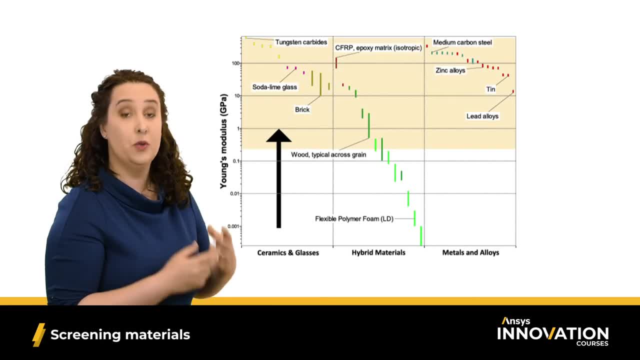 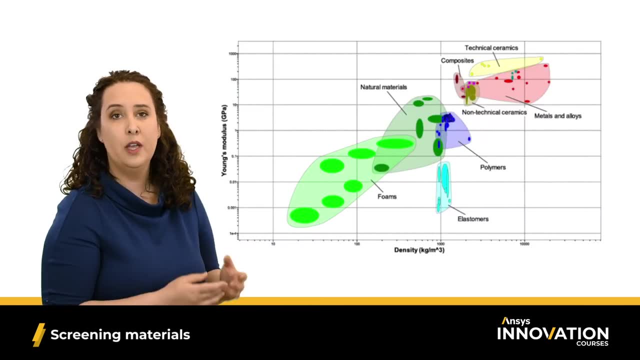 And now I can focus on ranking my materials that are left over to maximize my yield strength. So I'm focusing up here in my chart. I can also do this with bubble charts. Here we're really focusing on which of these four quadrants I want to have my material reside in. So let's say I'm shooting for this optimal. 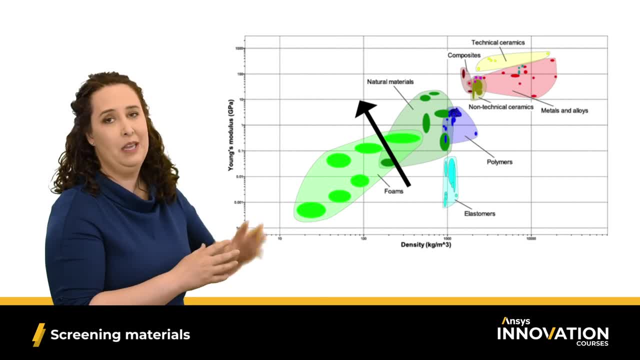 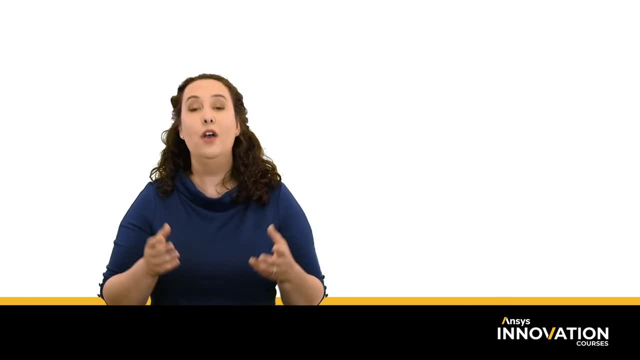 upper left-hand corner. So I'm simply going to focus all of my attention in this direction, And with that we've come to the end of our lesson. We've shown how we can take our material property charts and visually select materials, Using screening and ranking based on design criteria, In the final lesson for this course.